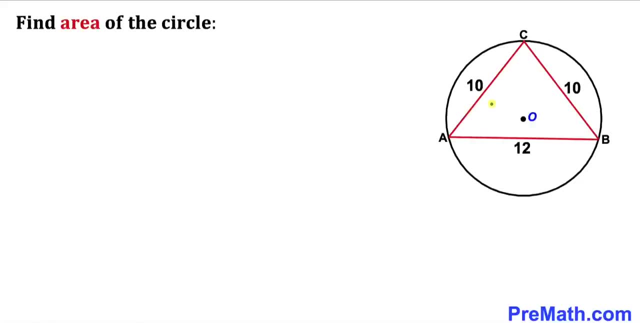 welcome to pre-math. in this video we have got this, an isosceles triangle, ABC, inscribed in a circle, as you can see in this diagram, such that this side length AC is 10 units, this side length BC is 10 units as well, and this side length AB is 12 units. and now we are going to calculate the area of this. 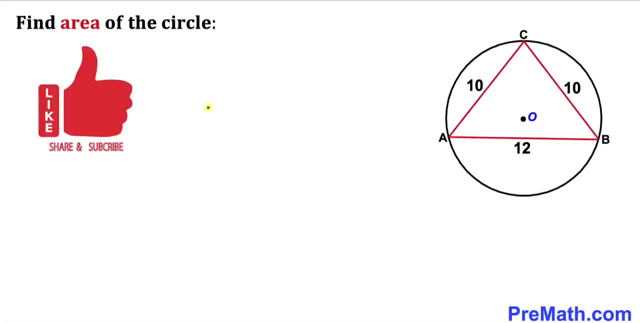 circle. Please don't forget to give a thumbs up and subscribe. Let's go ahead and get started with this solution. Here's our very first step. we know that we are dealing with an isosceles triangle. now let's go ahead and drop a perpendicular from this point C, so this is going to pass through. 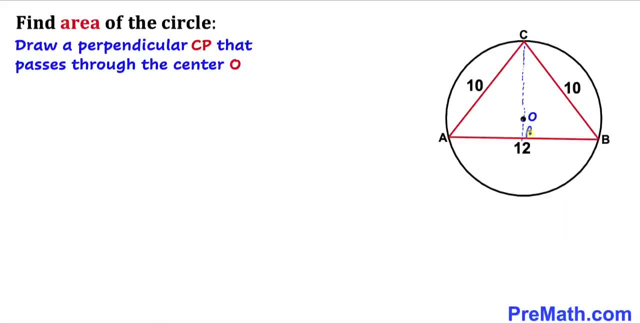 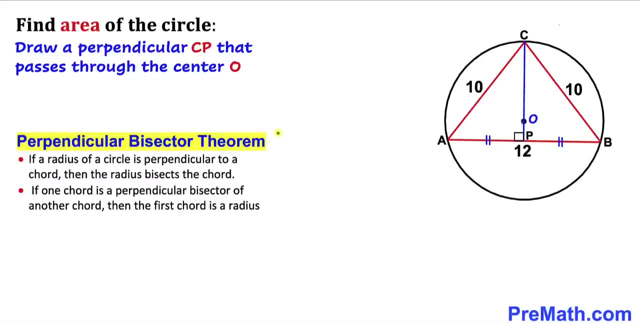 the center O, and this is our point P over here. and here's our much nicer looking diagram. now recall the perpendicular bisector theorem. according to this theorem, if a radius of a circle is perpendicular to a chord, then the radius bisects that chord. so therefore we can see that. 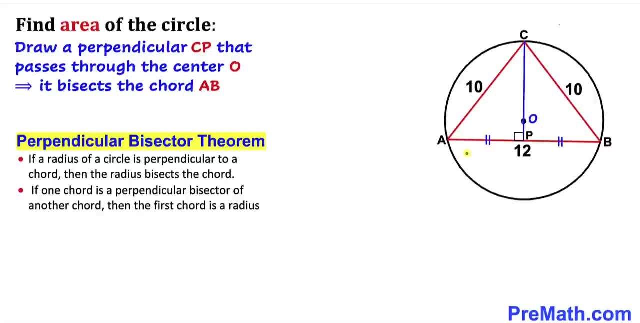 this perpendicular bisects this chord a- b into two equal parts: this part and this part. if this whole length is 12, so this side is going to be 6 units and this is going to be 6 units as well. so therefore, this side length a- p is 6 units. and here's our next step. let's focus on this triangle. 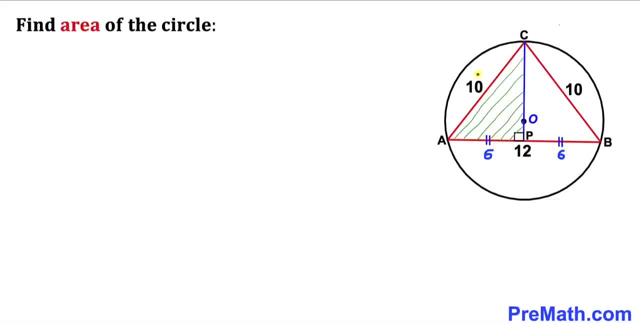 a, p, c. we can see that we have been given two sides: this is 10 units and this is 6 units. now we are going to calculate this side, c, p- and since we are dealing with our right triangle, therefore, we are going to use the pythagorean theorem. and here's our pythagorean theorem: a square plus b square equal to c square. 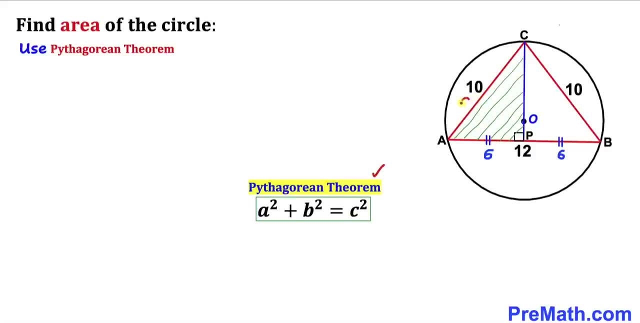 let me go ahead and call this longest leg as our side c. i'm going to call this horizontal side a and this vertical side b. let's go ahead and fill in the blanks in this pythagorean formula. in our case, a is 6, so this is going to become 6 square plus b. we don't know. let me just write on b square and c in our. 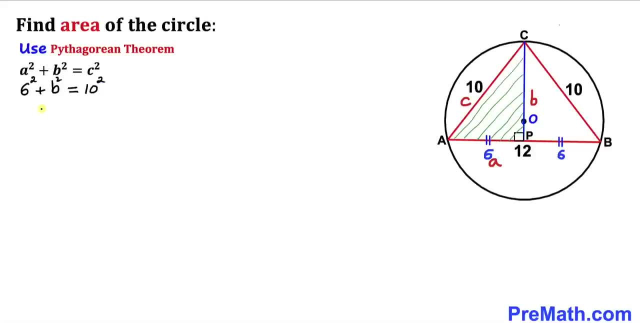 case is 10 square. so let's go ahead and simplify. 3 square is 36, plus b square equals to 100. let me go ahead and subtract 36 from both sides. we can see that this is gone. so therefore, our b square value turns out to be 64.. let's go ahead and take the square root 1 to this. 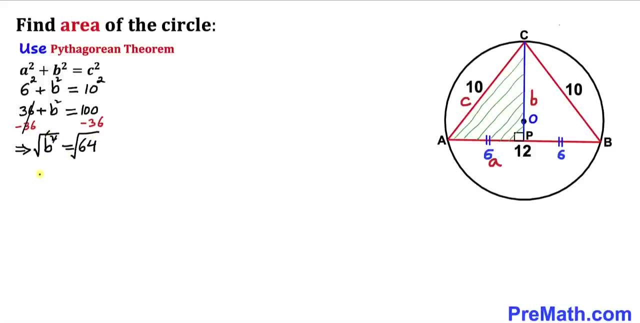 square. so this square and square root is gone. so our b value turns out to be positive 8. therefore, our this side b turns out to be 8 units. and here's our next step. we know that this c o, this is our radius, so let me go ahead and call this radius lowercase. 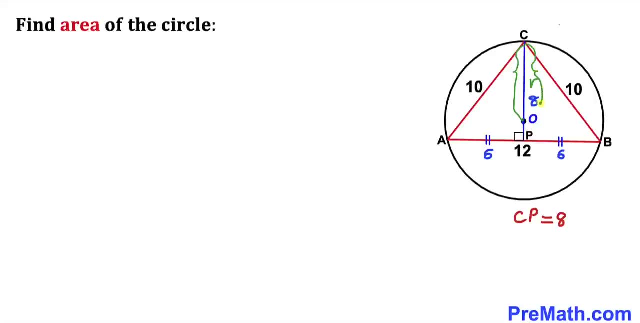 r and we know that this whole side length is eight units. so therefore, this side length o p is going to be simply 8 minus r. and here's our next step. let's go ahead and connect this point a with this center of. let me go ahead and illuminate this point again: 8 plus b, that's going to be 8.5, is going to be 0.8x. 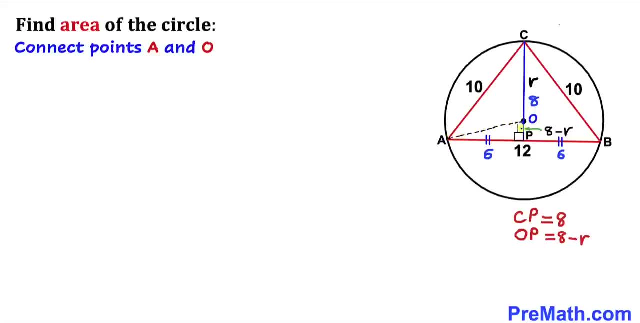 and connect this point. and here's our much nicer looking diagram. and now let's focus on this tiny triangle, APO. and we know that this is a right triangle. so therefore, we are going to use the Pythagorean theorem once again. and here's our Pythagorean theorem: a square plus b square. 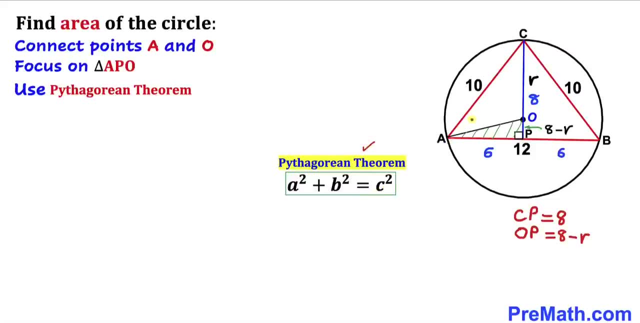 equal to c square. let me go ahead and call this longest leg as our side c. I'm going to call this horizontal side a and this side op. I'm going to call this side b. now we can see that this side length AO is nothing more than just the radius of this circle, so I'm going to call this: 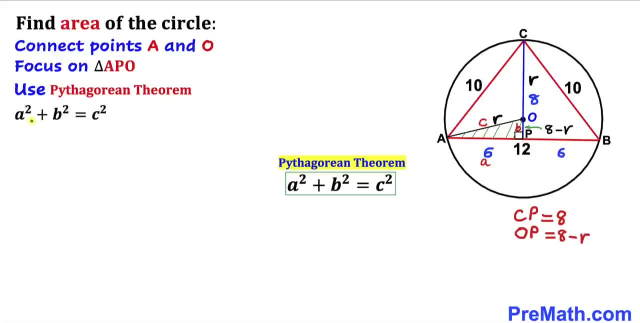 radius r as well. so let's go ahead and fill in the blanks in this Pythagorean formula. in our case, a is 6, b value is 8 minus r and c value is this radius r. therefore, our this equation is going to become 6 square plus b in our 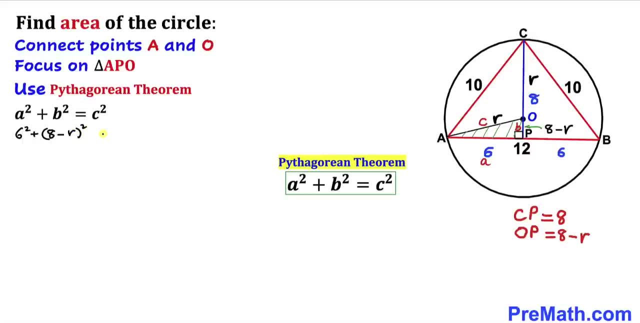 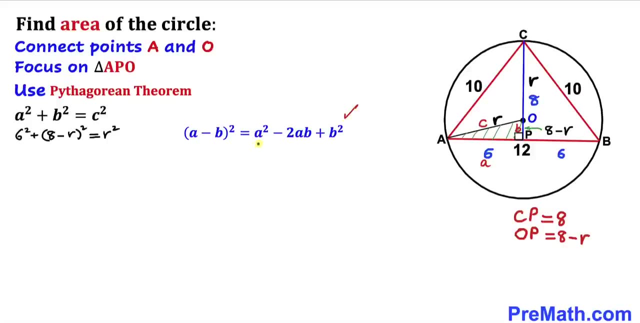 case is 8 minus r whole square equal to r square. and now let's recall this famous identity: a minus b whole square equal to a square. minus 2. ab plus b square. I'm going to apply on this part. therefore, we are going to have 6 square is: 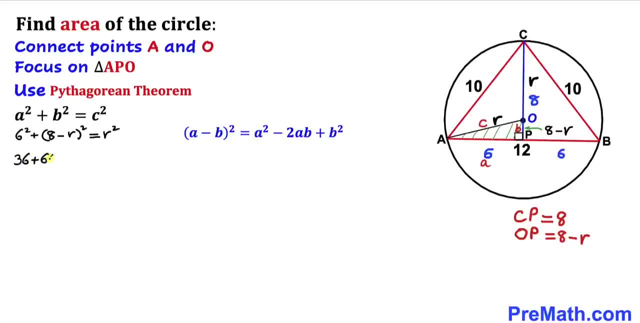 36, and this is going to become 64 minus 16 r plus r square, equal to r square on the right hand side. now we can see this: r square on the left hand side and r square on the right hand side. they are gone. let's go ahead and combine the like terms. that is going to give us 100 minus 16 r turns out. 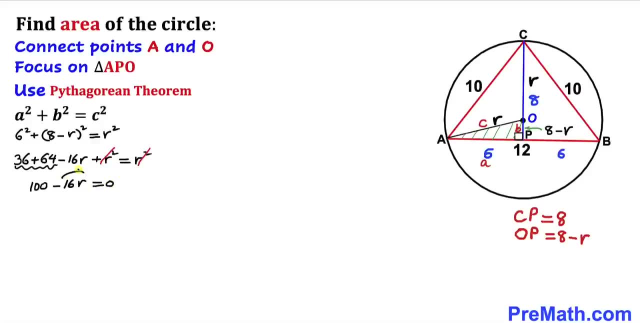 to equal to 0. let's move this negative 16 r on the right hand side, so we are going to get 16 r equal to 100. let's go ahead and divide both side by 16 now, so that means our r radius value turns out to: 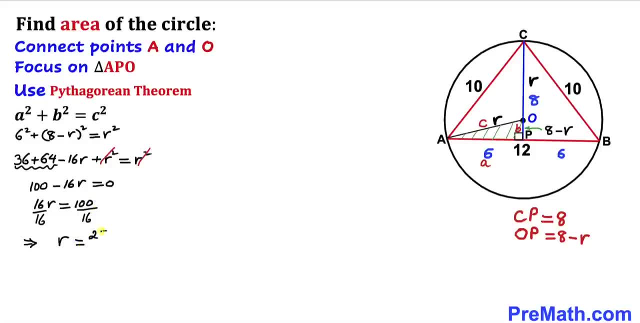 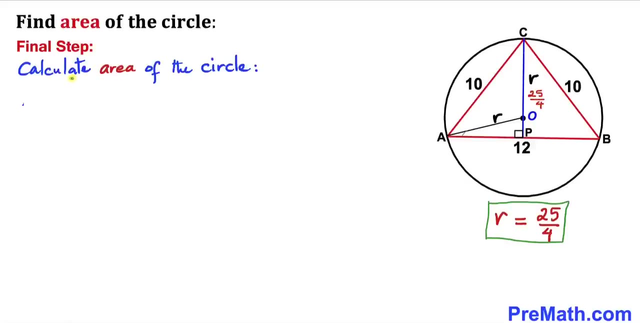 be. if we reduce the right hand side, that's going to give us a 25 divided by 4, and that is our radius. so thus our radius value turns out to be 25 divided by 4 units. and here's our final step. let's go ahead and calculate the area of this circle. now let's recall the circle of area formula. 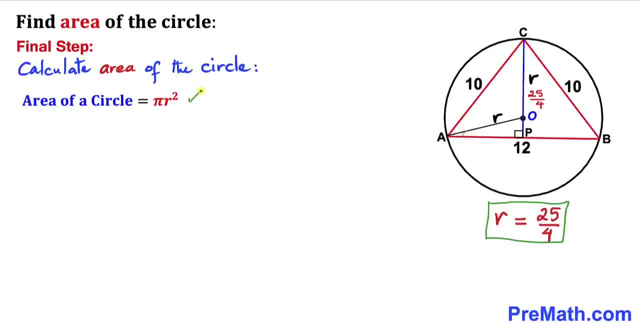 area equals to pi r square. in our case, our radius r is 25 divided by 4. now let's go ahead and fill it in. so this circle is going to be pi times r. in our case is 25 divided by 4 whole square. so if we